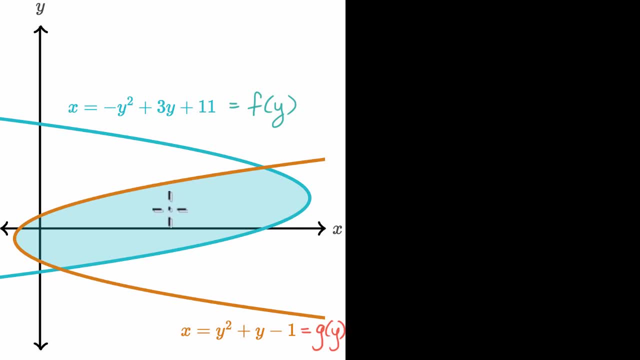 between these two curves, And I encourage you to pause the video and try to work through it All right. so a huge hint here is we're going to want to integrate, with respect to y, a definite integral where our bounds are in terms of y. 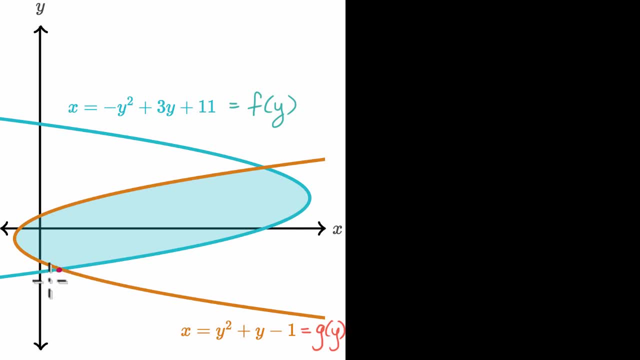 So, for example, this is this lower point of intersection right over here. This would be our lower bound in terms of y- Let's call that y one, And then this up here: this would be our upper y bound. So if we think about, where do these two curves intersect? 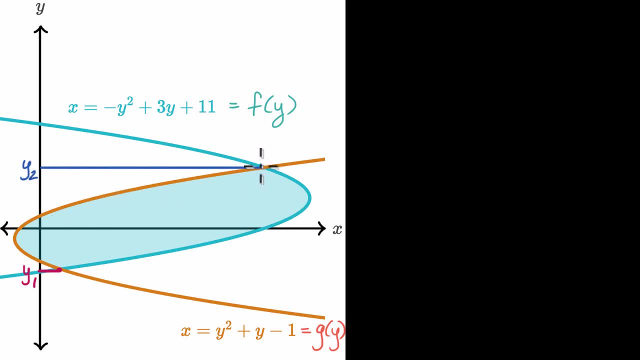 and we look at the y coordinates of those intersections. well, that gives us two nice bounds for our integral. So we're gonna take our integral from y one to y two, from y one to y two, y two. We're going to integrate with respect to y dy. 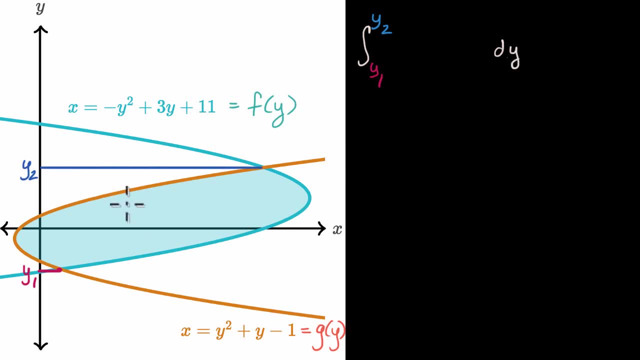 And so what are we going to sum up? Well, when we integrate, we can think about taking the sum of infinitely thin rectangles, And in this case it would be infinitely flat rectangles, since we're thinking about dy, So dy would be the height of each of these rectangles. 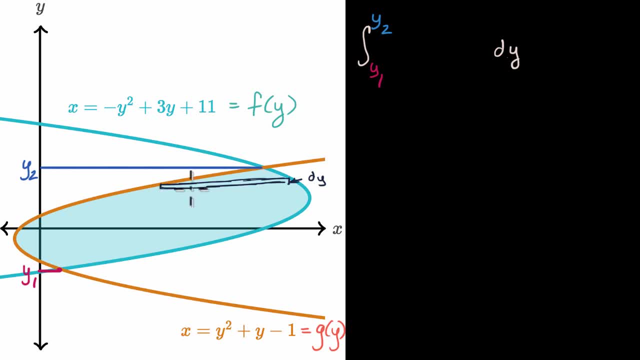 And what would be, in this case, the width or the length of this rectangle right over here? Well, over this interval from y one to y two, our blue function f of y takes on a weight of well y one, y two. 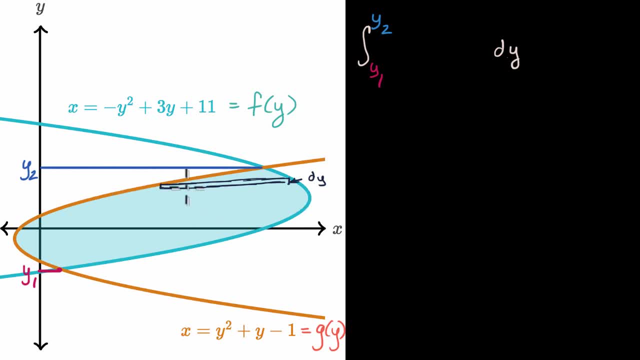 It takes on larger x values than g of y. So this length right over here, this would be f of y, f of y, this x value minus this x value minus g of y. So this is going to be f of y minus g of y, g of y. 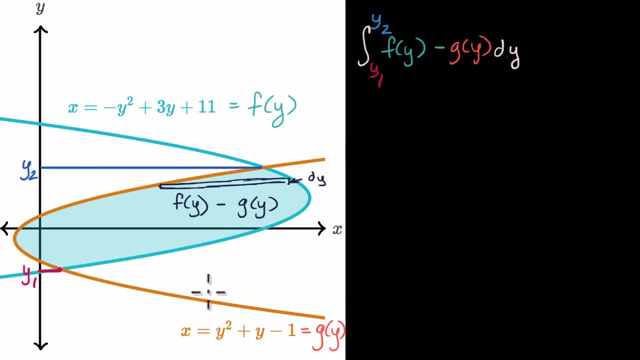 Well, we know what f of y and g of y are. Really, the trickiest part is is figuring out these points of intersection, Figuring out where these two curves intersect. They are both equal to x, so we can set these two y expressions equal to each other. 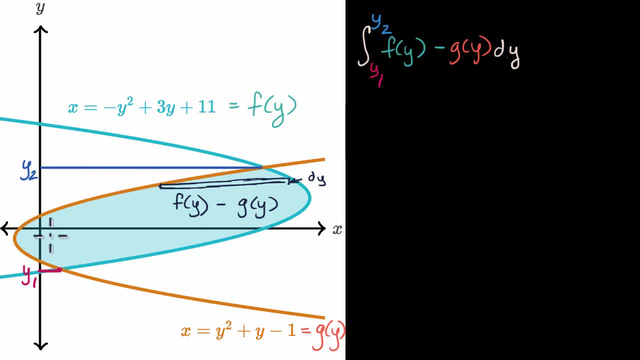 So we know that negative. let me do it in that other color. So we know that negative. y squared plus three, y plus 11 is going to be equal to: this is going to be equal to y squared plus y minus one. So let's just subtract all of this from both sides. 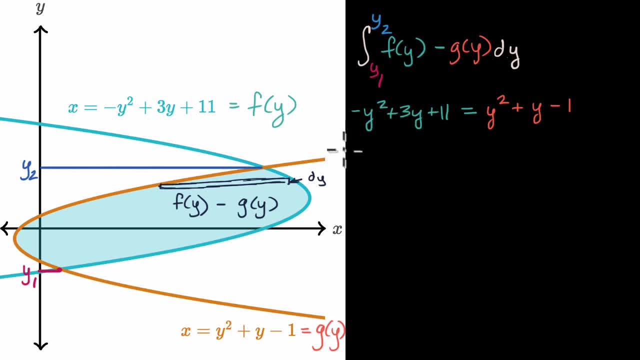 so that on the right side we have a zero and on the left side we just have a quadratic. So let's subtract y squared, Let's subtract y and then subtract negative one, which is just adding one. And over here we're going to do the same thing. 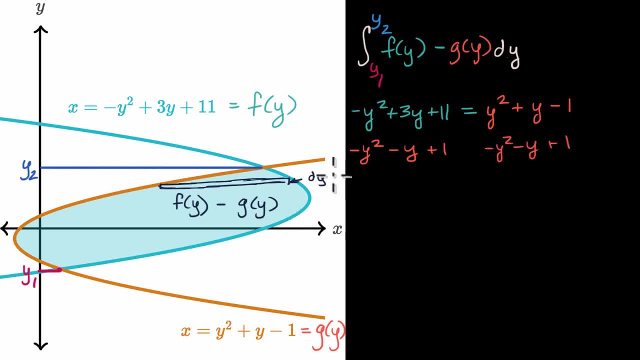 Minus y plus one, And what we are left with is going to be, hopefully, a straightforward quadratic. So let's see, this is going to be negative: two y squared plus two y. Am I doing that right? Yeah, plus two y plus 12.. 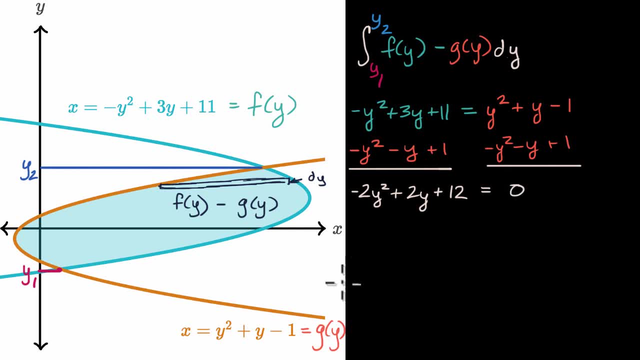 Plus two. y plus 12 is equal to zero. And then this over here I can factor out a negative two And I get negative two times y squared minus y minus six is equal to zero. This we can factor from inspection. What two numbers when we add equal negative one. 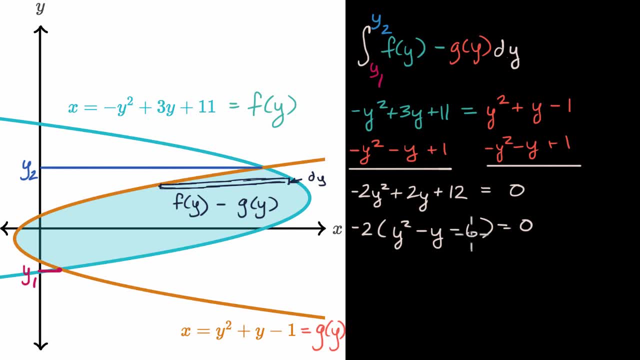 when we take their product, we get negative six. Well, that would be negative three and two. So this is going to be negative two times y minus three times y plus two. So this is going to be negative three and two. That's just straightforward, factoring a polynomial. 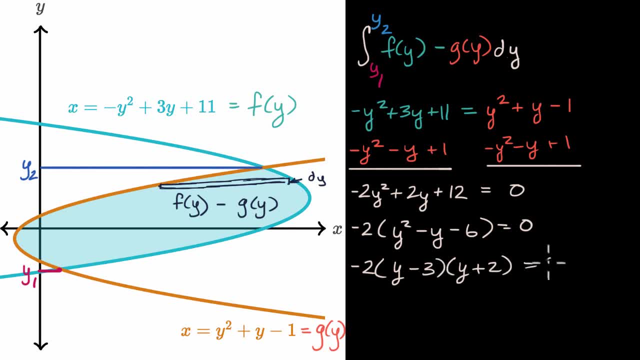 a quadratic- Did I do that right? Yep, that looks right- Is equal to zero. So what are the points of intersection? The points of intersection are going to be: y is equal to three and y is equal to negative two. So this right over here is: y is equal to negative two. 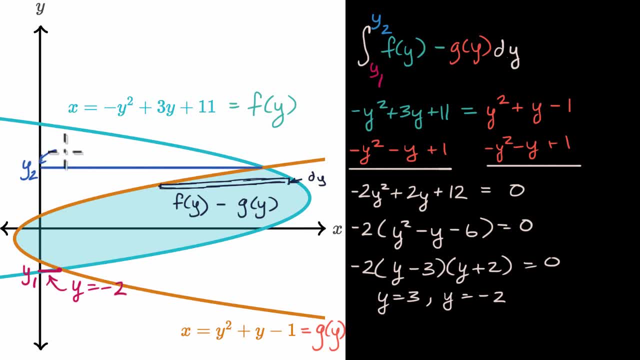 And then the upper bound is: y is equal to three. So now we just have to evaluate this from negative two all the way until three. So let's do that. I'm going to clear this out, so I get a little bit of real estate. 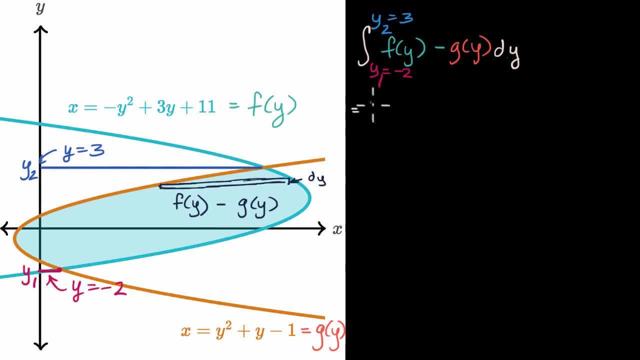 So this is equal to the integral from negative two to three of negative y squared plus three, y plus 11, minus all of this stuff. So if we just distribute a negative sign here, it's minus y squared minus y squared Minus y plus one, and then we have a dy dy. 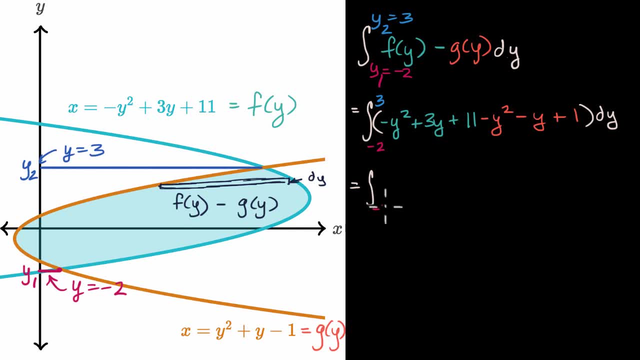 This is equal to the definite integral from negative two to positive three of. let's see negative y squared minus y squared. negative two, y squared, and then three, y minus y is going to be plus two y, and then 11 plus one plus 12.. 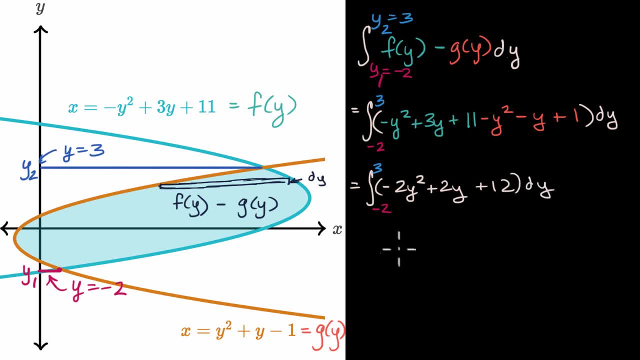 We saw this just now when we were trying to solve for y dy, and so what is that going to be equal to? Well, we just take the antiderivative here. This is going to be- let's see- negative two. 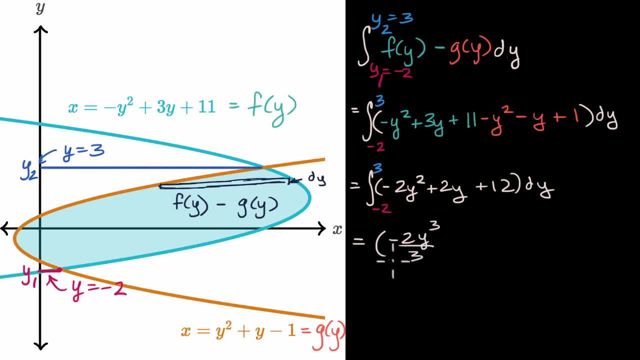 let's increment the exponent y to the third divide by that exponent reverse power rule, plus two y squared divided by two, which is just y squared, just the reverse power rule, and then plus 12y And we're going to evaluate that at three and at negative. 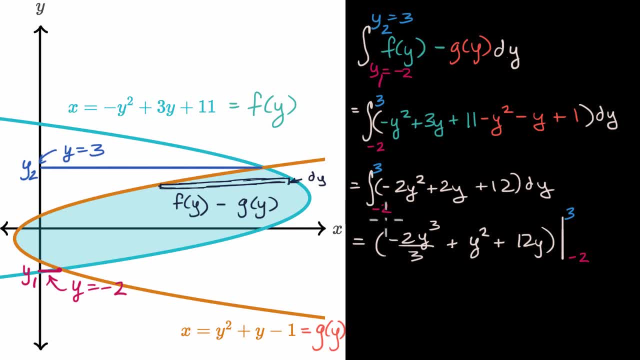 Negative two. So if we evaluate that at three, we are going to get, let's see, negative two times 27 over three plus nine plus 36, and then we are going to want to subtract minus all of this, evaluated at negative two. 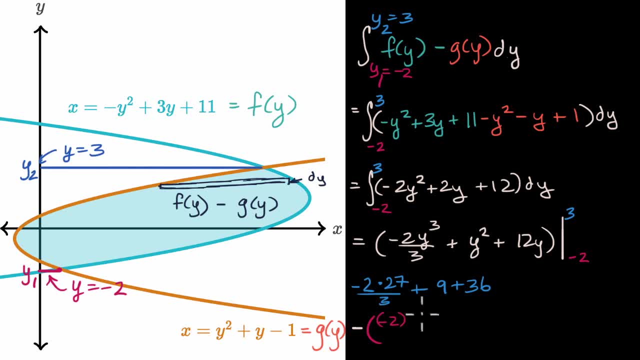 So it's going to be negative two times negative: eight over three plus nine plus 36.. Negative four minus 24, so we just have a little bit of mathematics ahead of us. So let's see, This is going to be: 27 divided by three is nine. 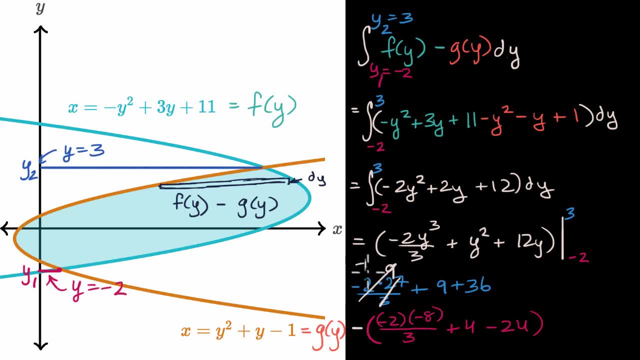 So this is negative 18, negative 18 plus nine is going to be negative nine plus 36.. All of that is going to be equal to: so the stuff in blue is equal to 27,. right, Did I do that, right? 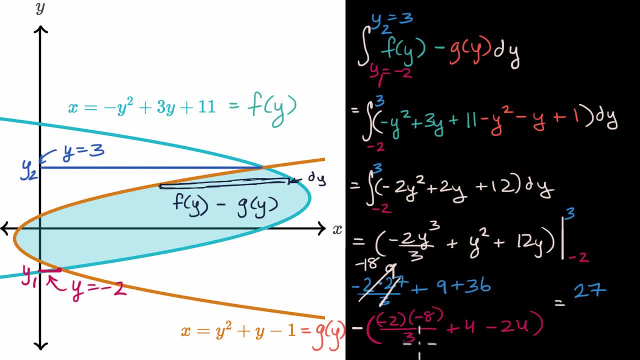 Yeah, negative, 18 plus nine, yep 27.. And then all of the stuff in red over here we have. this is going to be negative times a negative. So it's 16 over three plus four minus 24.. 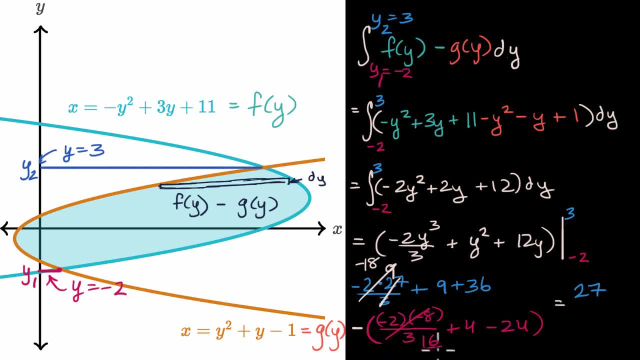 So that is going to be 16 over three and then minus, minus 20, minus 20.. But then we have this negative out here. So it's: if we distribute that we'll get plus, 20, minus. we could say, instead of 16 over three we'll get minus 20..